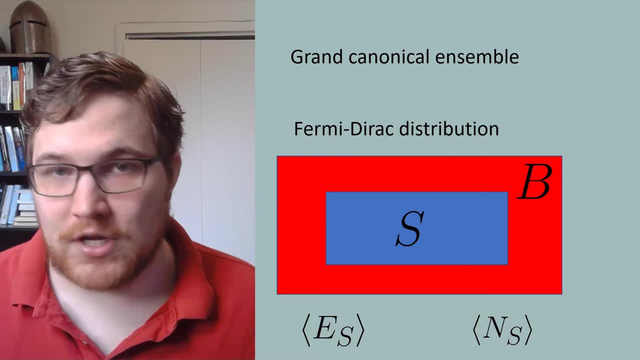 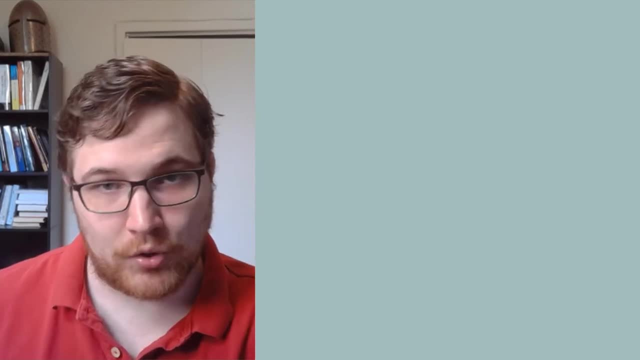 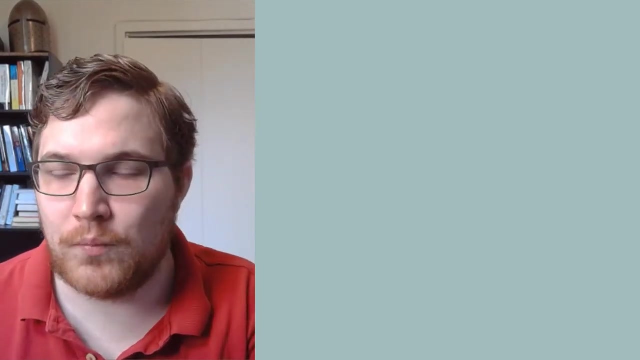 bath is there. This is just for notational convenience. If you're a frequent viewer of this channel, you'll know that this situation is quite familiar to us. In the video on the principle of maximum entropy, we discussed the scenario when we were embedded in a bath. 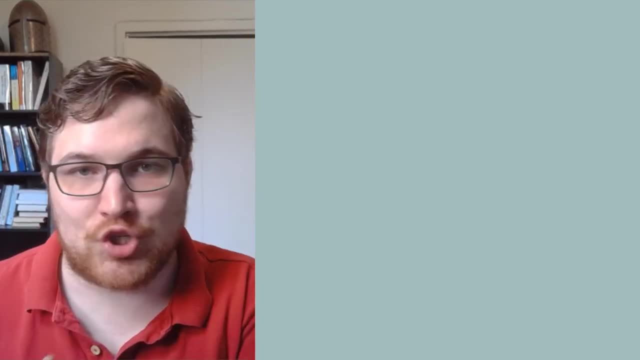 where the energy was constantly overloaded. sekarang We synchronously drop the subscript S for our system and then just assume that the bath is there. This is just for notational convenience could be exchanged between the system we were studying and the bath itself. so we 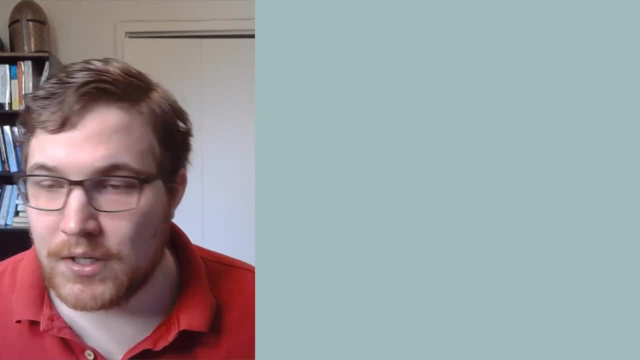 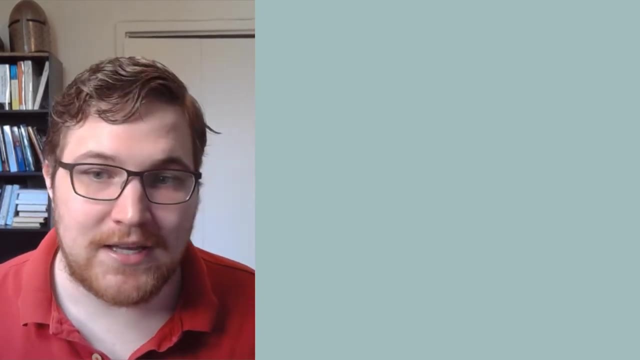 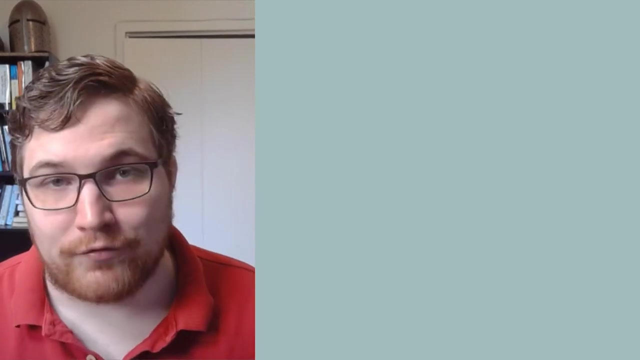 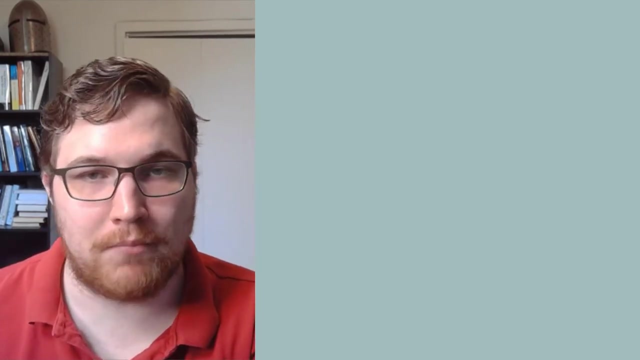 can appeal to Jane's principle of maximum entropy again to find the probability distribution that best describes our current situation, given our limited information, from the macroscopic information that we might be provided, that is, the average energy and the average particle number of our system. so we assign a probability P to each microstate of the system which we 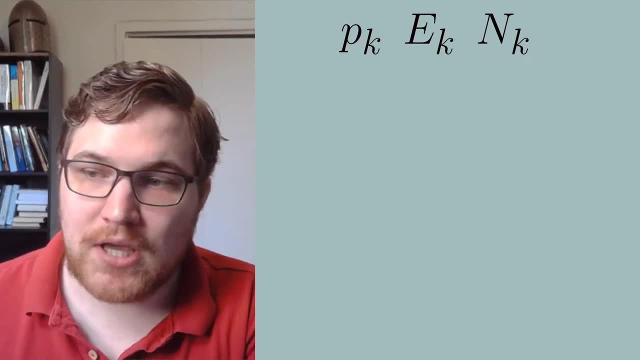 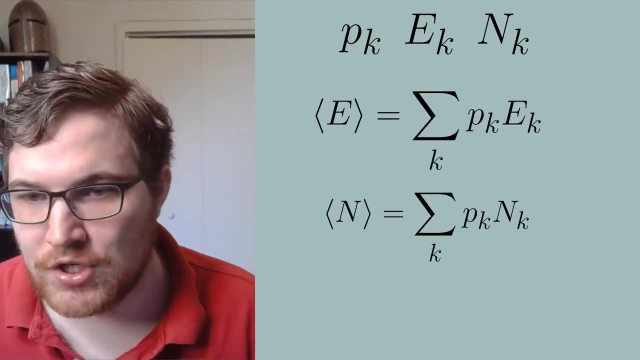 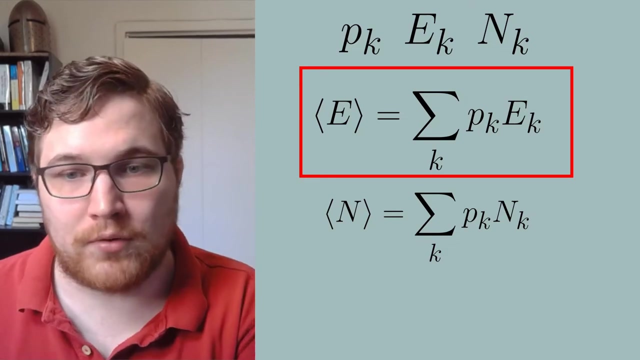 label by an index K, and at each K we have a corresponding energy and particle number. we define the expected value of energy for our system in terms of these probabilities, where the sum is over all microstates. we similarly define the the expected value of the number of particles in our system. 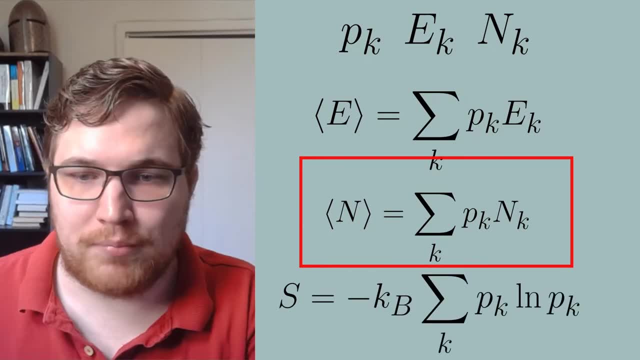 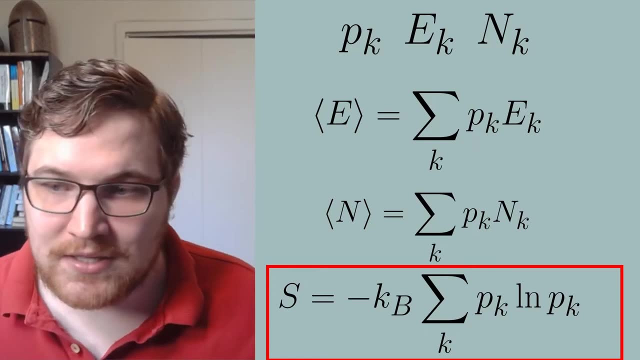 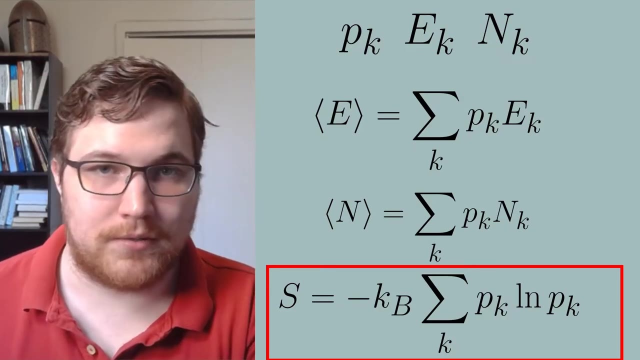 system. As always, we have the entropy S defined in terms of the probabilities themselves that we're looking to find, and this is the quantity we want to maximize. with constraints coming from the energy and the particle number of our system, The principle of maximum entropy tells us to solve. 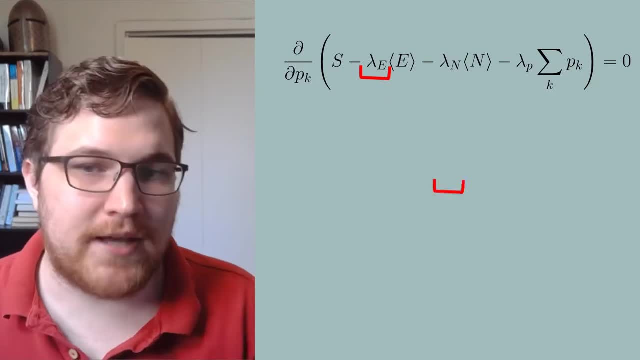 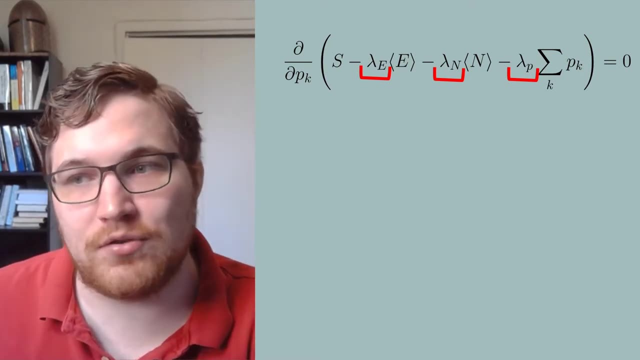 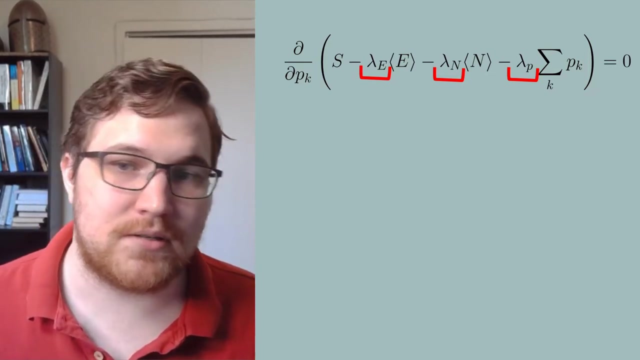 the minimization problem written here. The lambdas are Lagrange multipliers, as usual, and the final term in the expression forces us to find a normalized probability distribution, that is, that all of the probabilities sum up to one. Performing this minimization tells us that 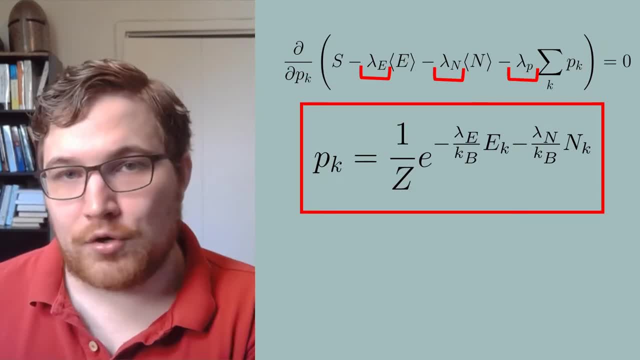 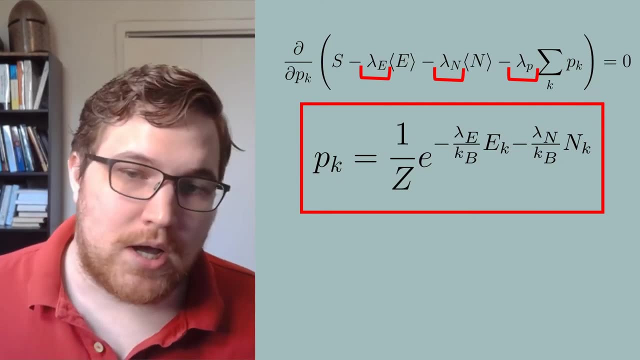 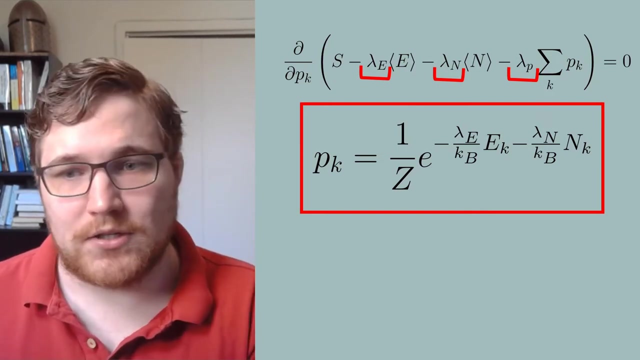 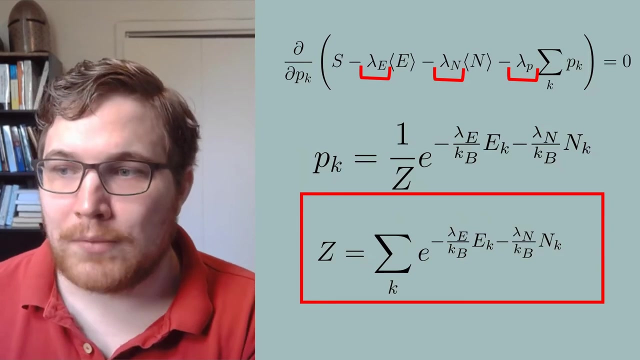 the probabilities look a lot like the thermal distribution or the canonical distribution from before, just with the inclusion of the extra particle number property of our microstates. We call this distribution the grand canonical ensemble, and the partition function z is defined as usual. normalizing the probability distribution: As usual, we need to go back to thermodynamics. 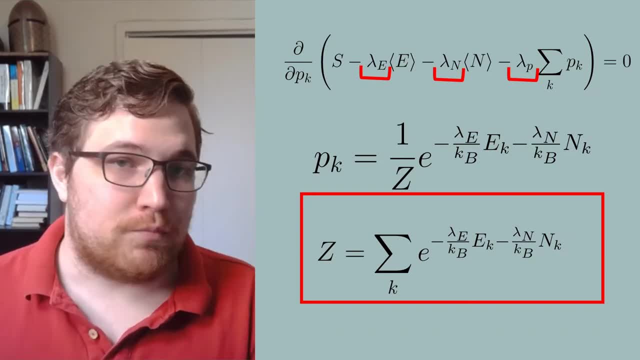 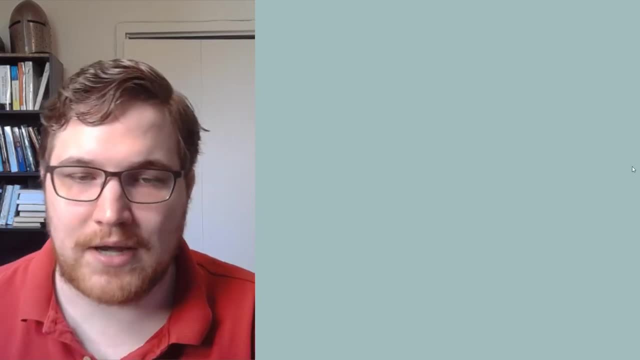 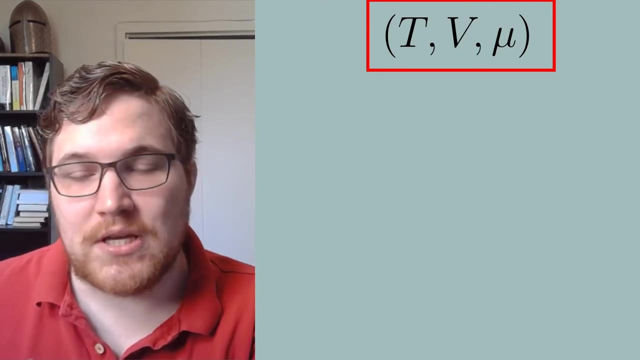 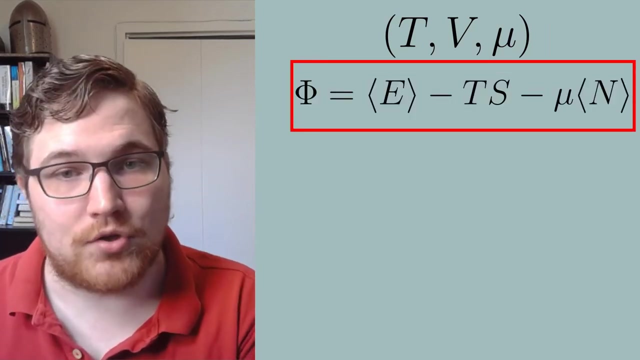 to figure out what our Lagrange multipliers actually represent In thermodynamics. we have a thermodynamic potential with natural variables: temperature, volume and chemical potential. This free energy is called the grand potential and is written as a Legendre transformation of the average energy. Equilibrium exists when this potential is. 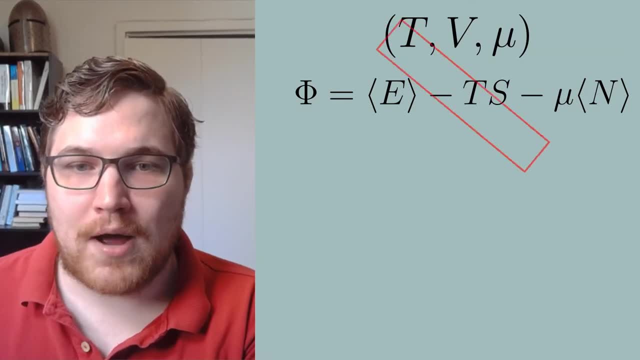 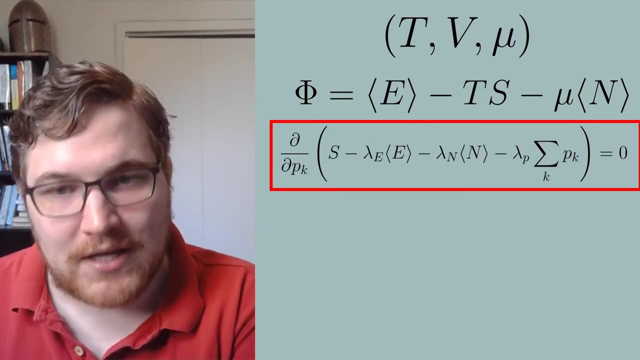 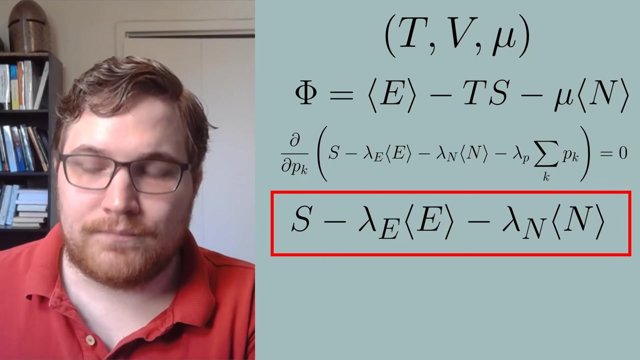 minimized and, interestingly for us, we can view our maximum entropy principle as equivalent to the minimization of this potential. I won't go over this argument in completion, but you should be able to see that when you look at the grand potential and you look at the function, 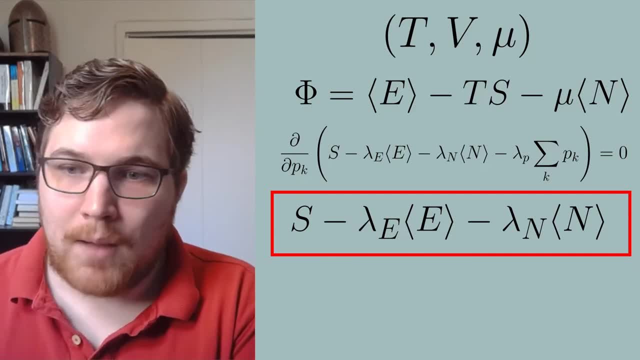 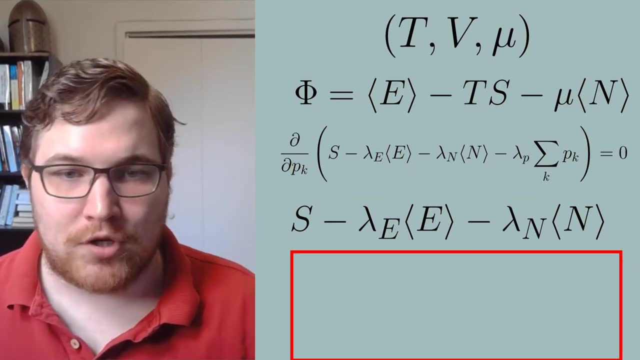 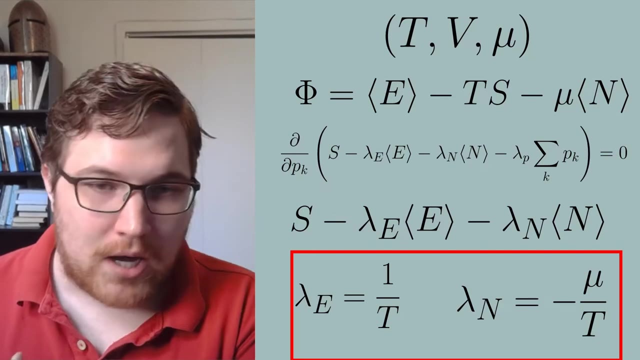 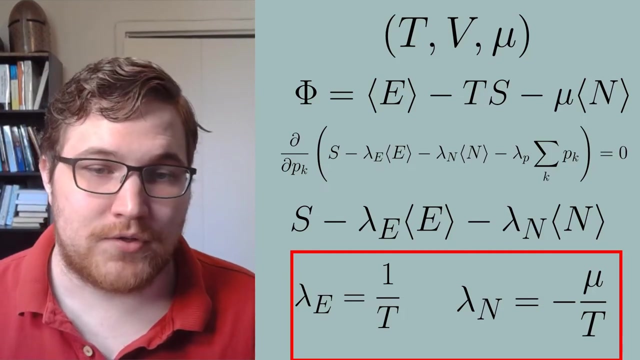 we are maximizing, with its constraints, that this leads to equivalent extremization principles if the following expression between the Lagrange multipliers and temperature and the chemical potential are satisfied. So if this is true, then we have identical extremization principles, and this relates our Lagrange multipliers to physical parameters. 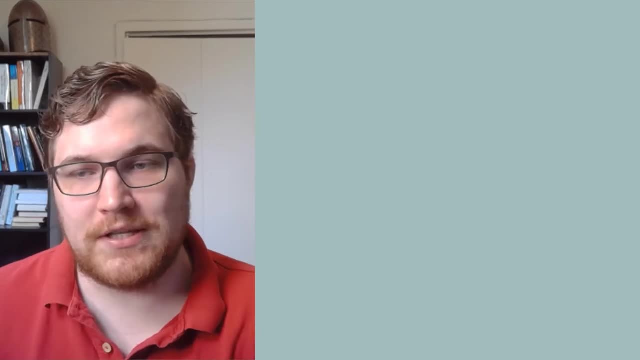 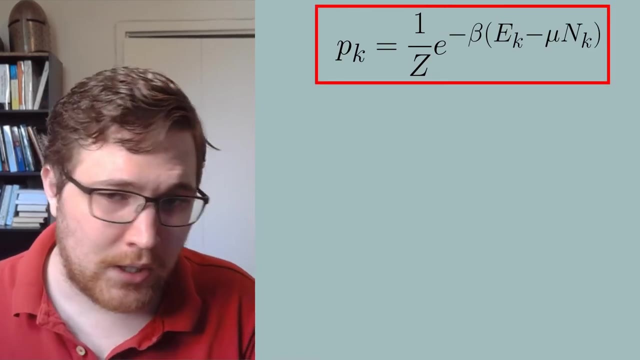 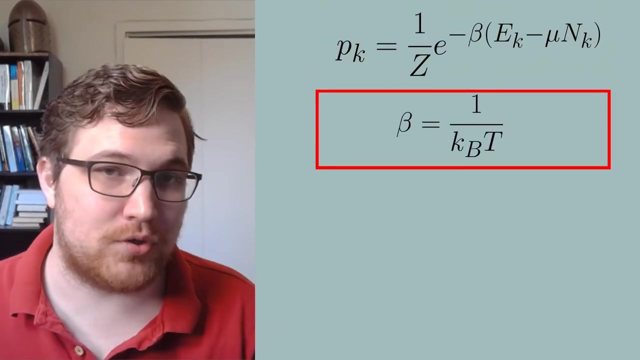 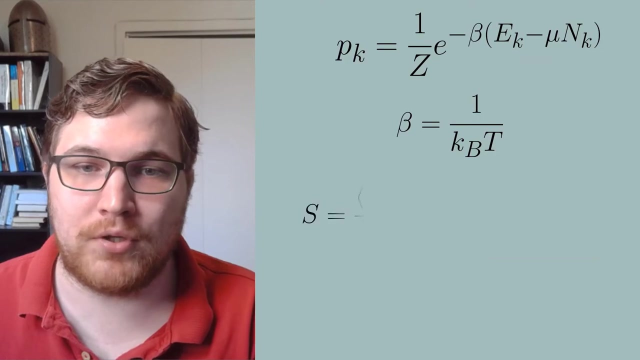 So, to summarize, our probability distribution is related to the temperature and chemical potential, as the following expression: where we have defined beta as 1 over the Boltzmann constant times, the temperature. Plugging this distribution into our definition of entropy tells us how to relate this probability distribution back to the grand potential Reorganizing gives. 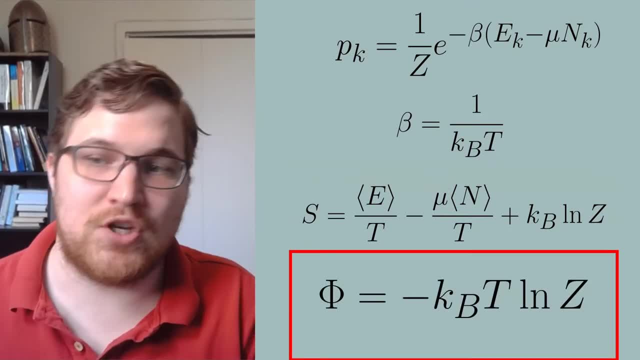 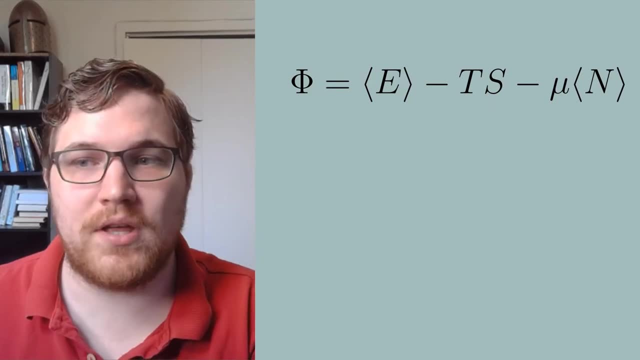 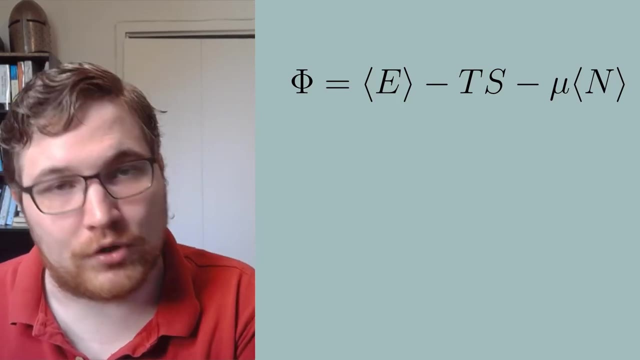 us the expression for the free energy in terms of the partition function. Back to our definition of the grand potential. we know that it is a Legendre transform of the energy. so we get the following relation for small changes in the potential. This allows: 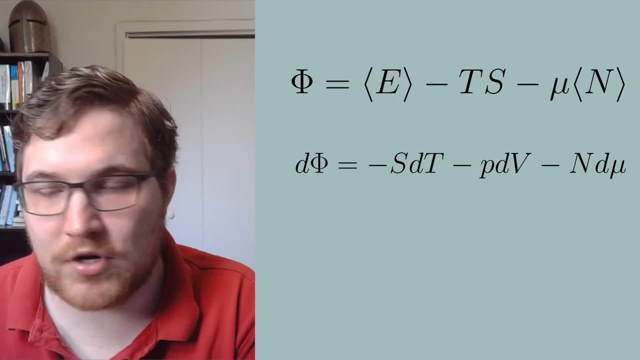 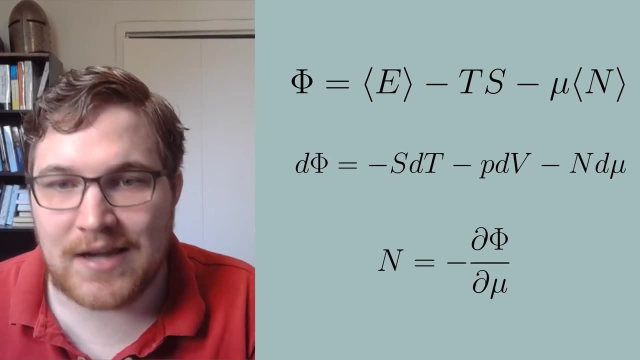 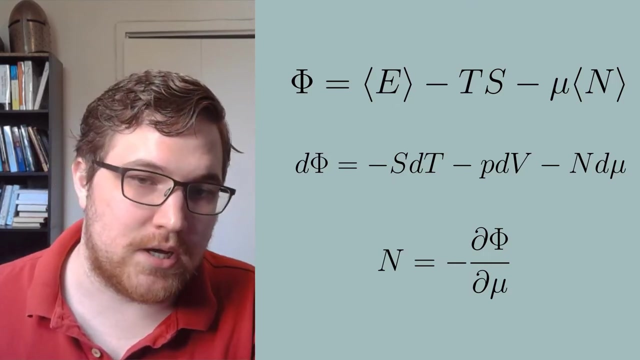 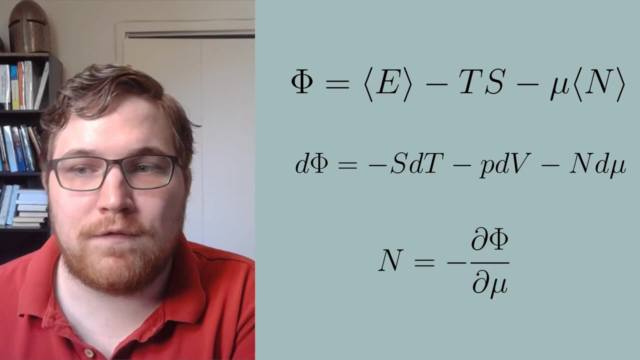 us to read off formulas for the entropy pressure and particle number, For example. the particle number is defined as the negative of the partial derivative of the potential with respect to the chemical potential, Just like our video on the canonical partition function. we therefore consider: 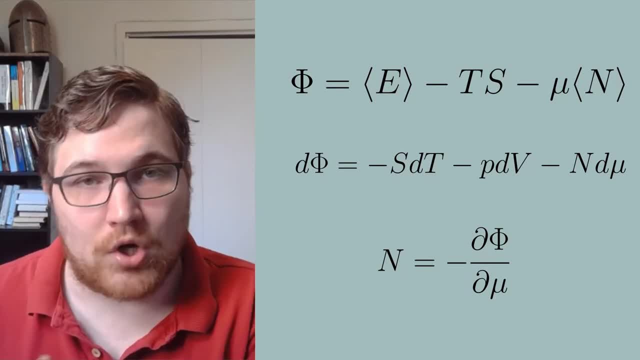 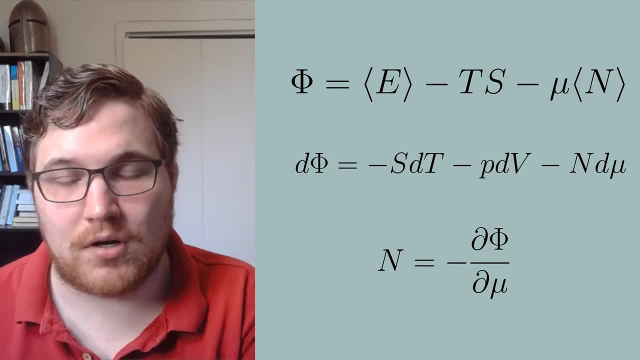 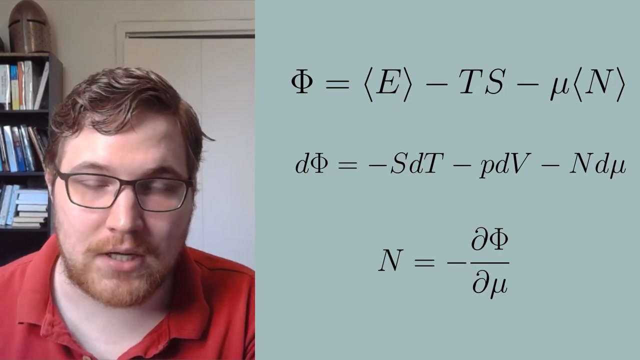 a problem solved with the grand canonical unsolved function for the chemical part释個有 terrific symbol if we can exactly evaluate the grand canonical partition function and recover the grand potential. This gives us access to anything we might be interested in about our system. 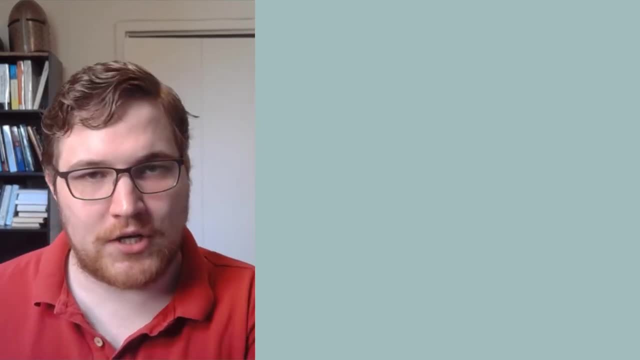 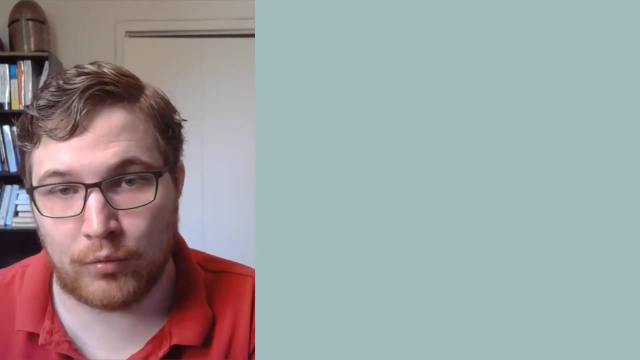 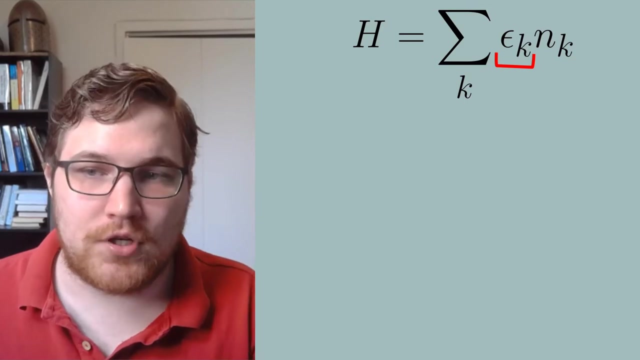 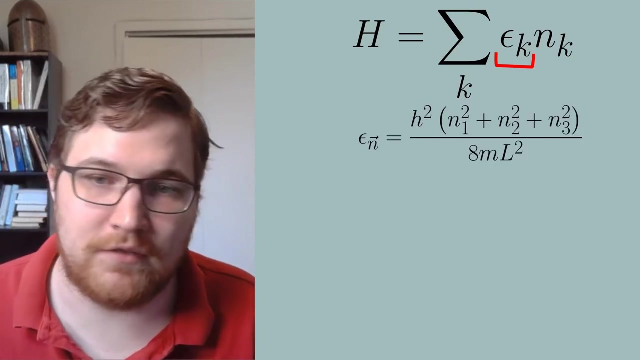 So now let's focus our attention on a problem of electrons or, more generally, fermions, described by the following: Hamiltonian Epsilon with the label K is a single particle energy. In the case of an ideal gas, for example, as we've seen before, the label K could be a vector of positive integers. 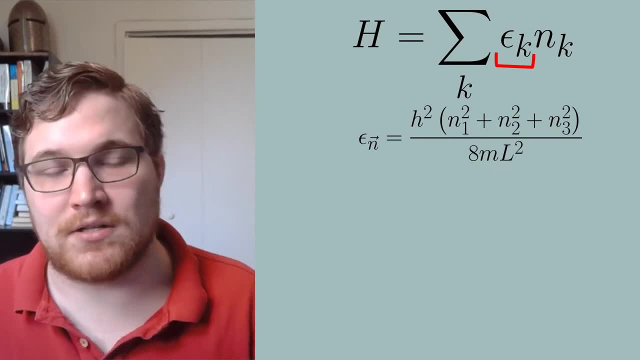 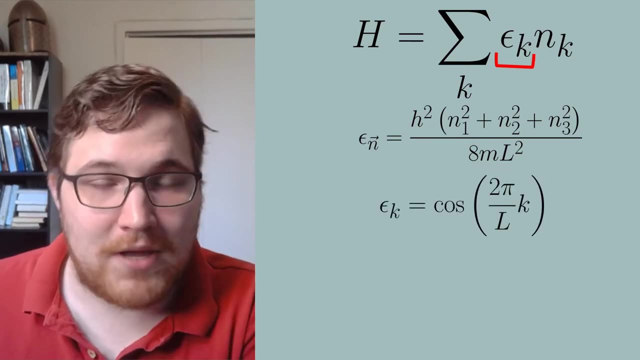 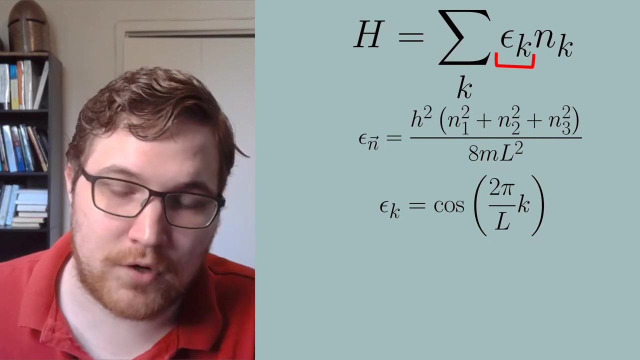 defining the energy of an electron in a box of side length L. We could also consider fermions hopping on a lattice in, say, one dimension with L total lattice sites And our single particle energies would be written as a cosine function, where K is just some integer. 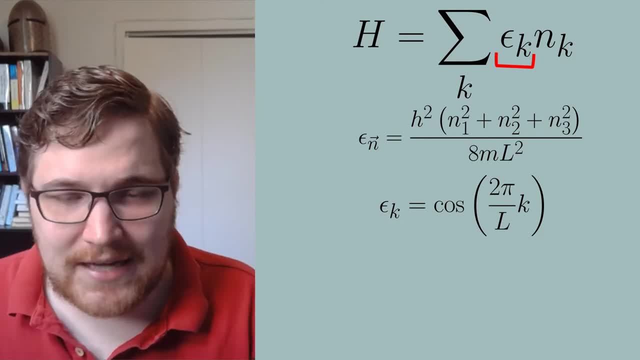 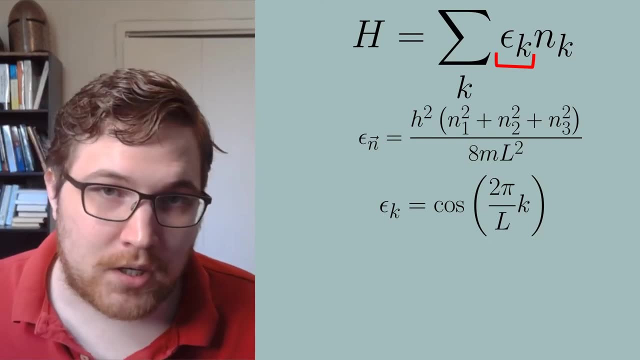 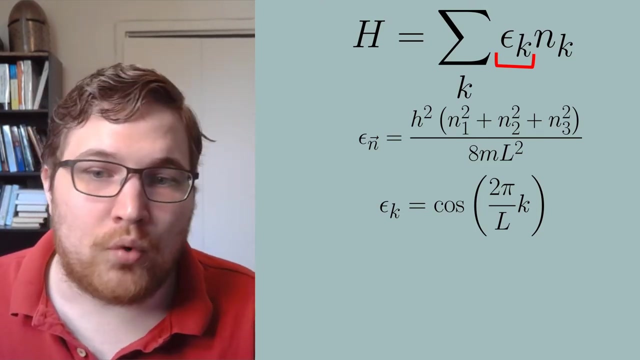 from one to L. The NK is special here, It's the number of fermions in a state K. Since we are considering fermions in this example, then for each microstate label K we can only have zero or one fermion in that microstate. 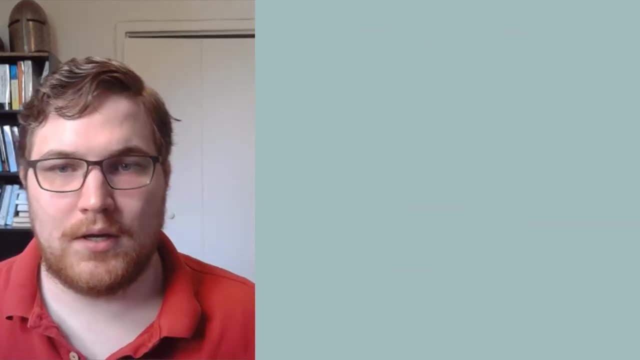 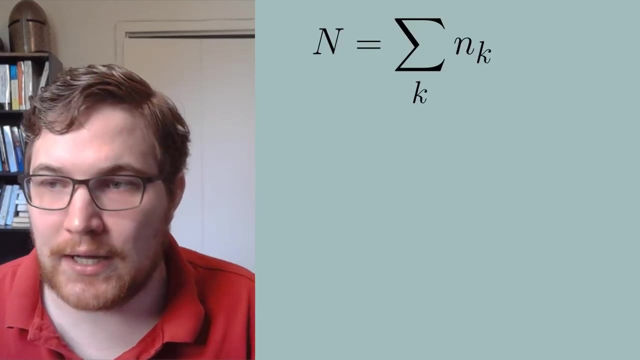 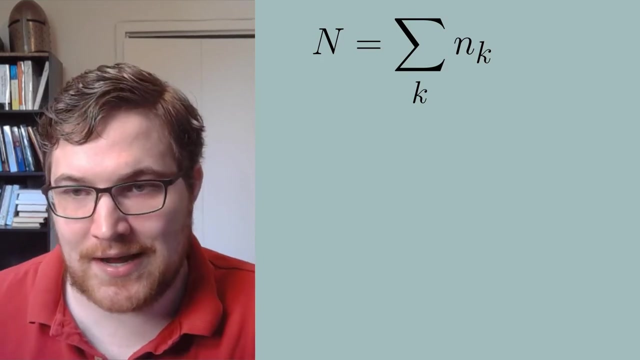 This is due to the Pauli exclusion principle. The total number of particles in our system is written in terms of the occupation numbers, little n, subscript K, So it's just a sum over these numbers. The microstates that tell us our energy and the total number of particles are therefore: 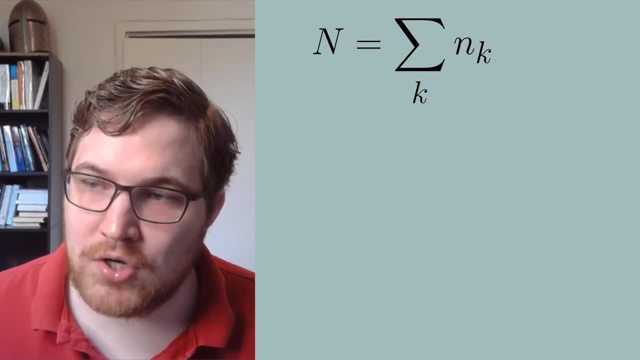 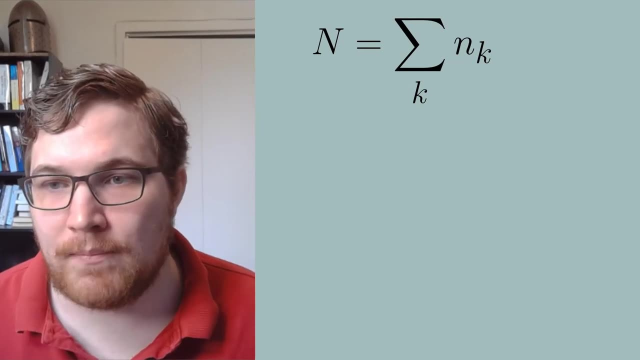 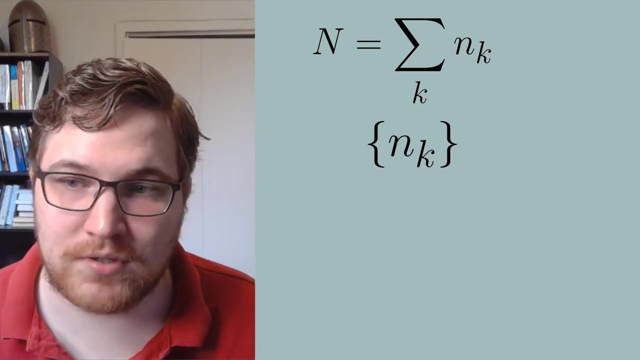 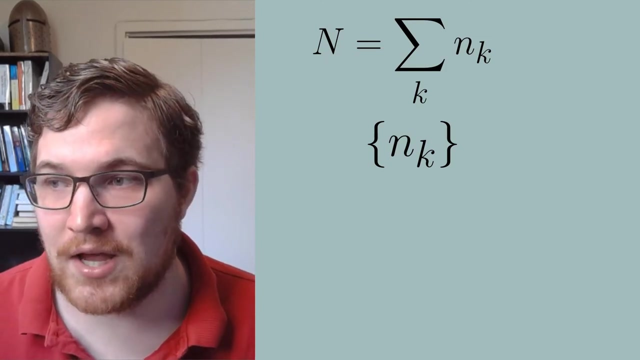 fully described by a set of occupation numbers- N, subscript K For each K, where each occupation number can be either zero or one. So we write a specific configuration or a specific microstate then by this curly bracket notation that tells us that it's a collection of zeros, and ones for each label K. It's then interesting to ask the question. 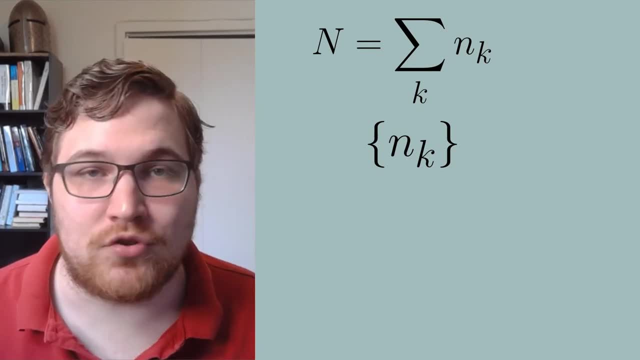 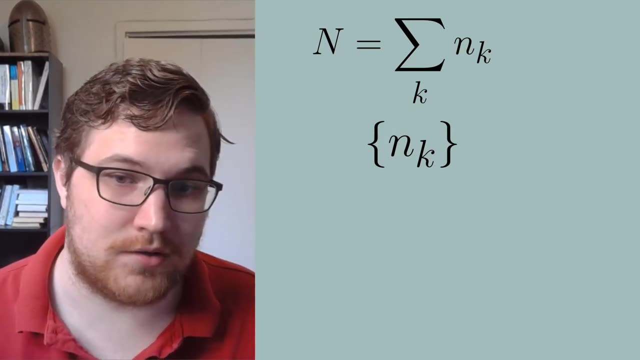 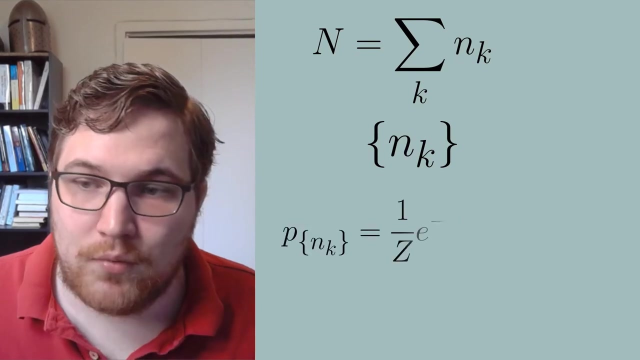 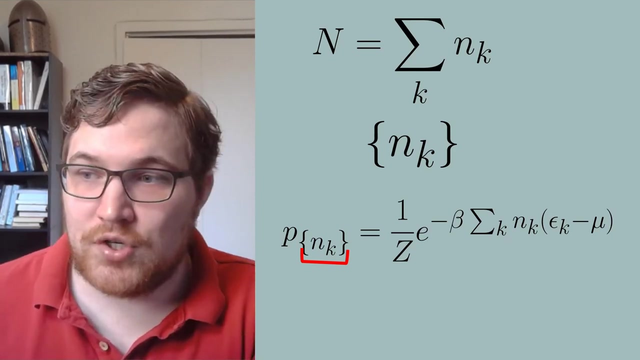 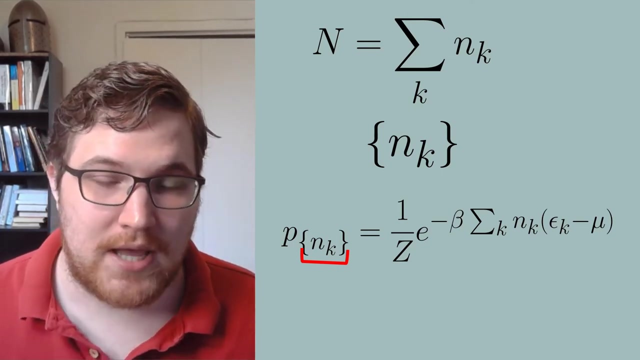 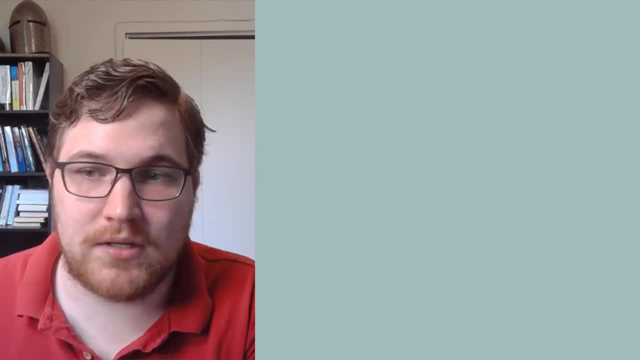 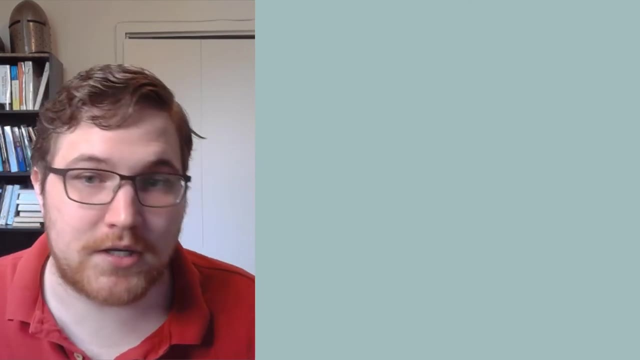 % 80.. % 80.. % 80.. € 100.. € 100.. interested in the properties of one occupation number, we can first split the expression for the probability up into a product of parts where each part only takes into account one. 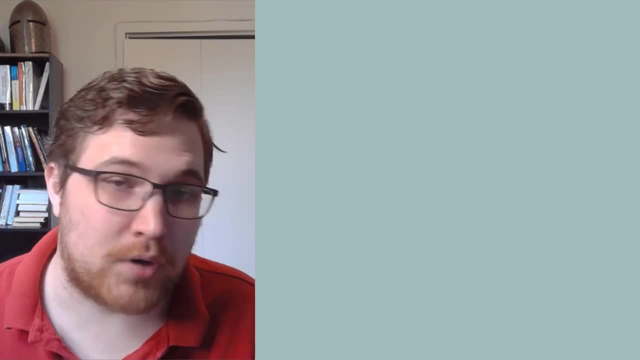 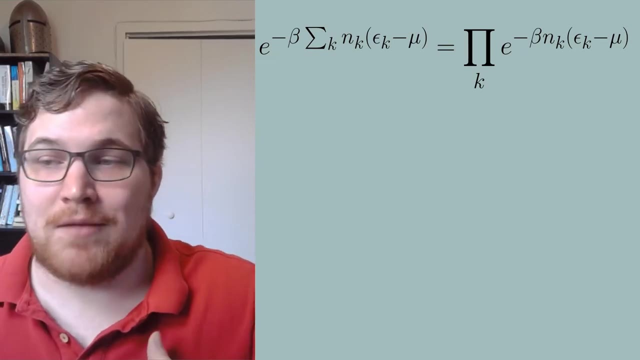 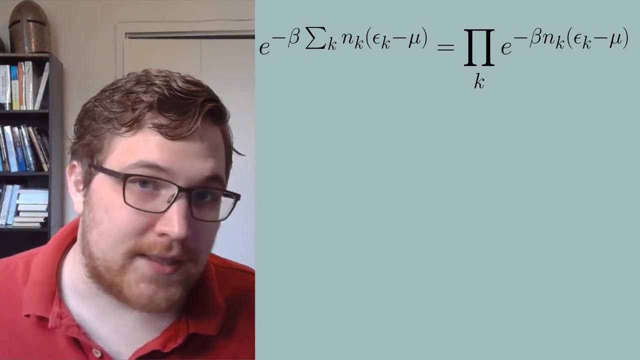 occupation number. Looking at the numerator of the probability first, we can re-express the sum in the exponential instead as a product over each individual occupation number. So then now we need to look at the partition function. We use the same factorization as above and write our expression. 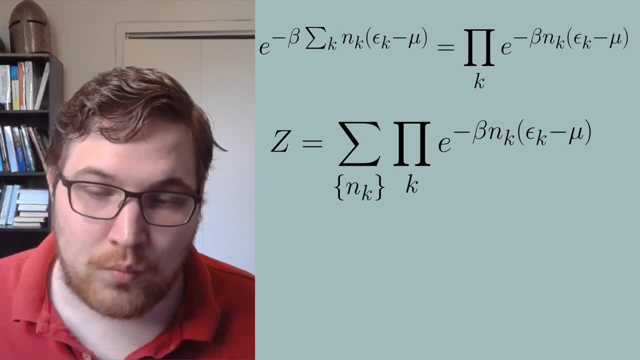 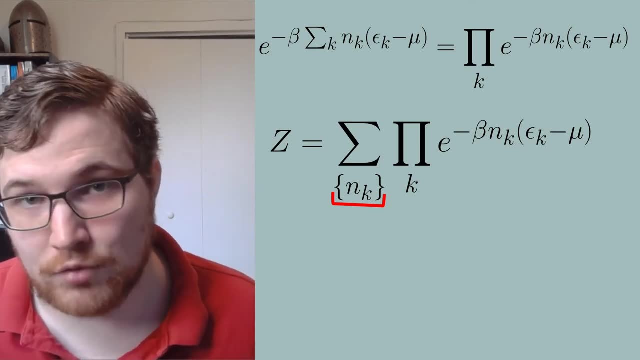 as the following: The sum, here with the curly braces and the occupation numbers, is telling us to sum over all possible sets of occupation numbers or all possible sets of minuses. So we can use the same factorization as above and write our expression as the following: 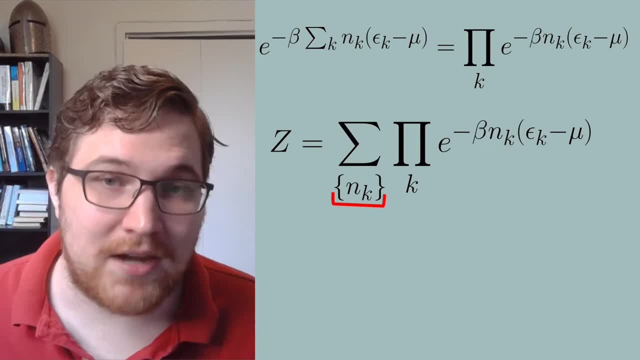 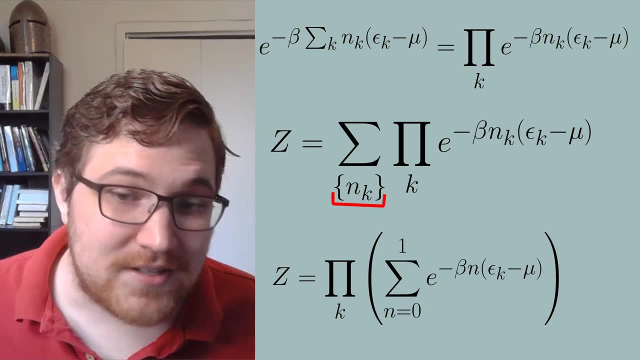 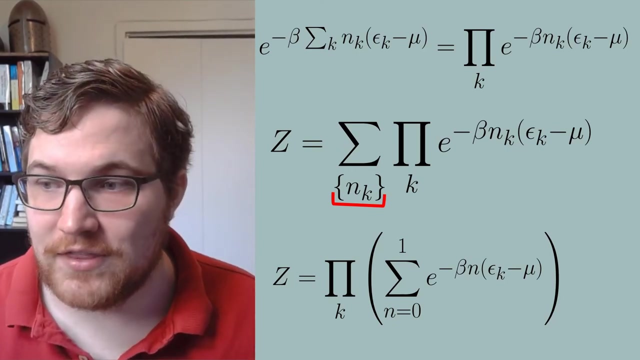 To put this into an independent form as well. we interchange the sum and the product in the following way: If this isn't immediately obvious how to do this, that's totally fine. Try to write it out by hand and convince yourself that this step is correct. Looking at the partition function. 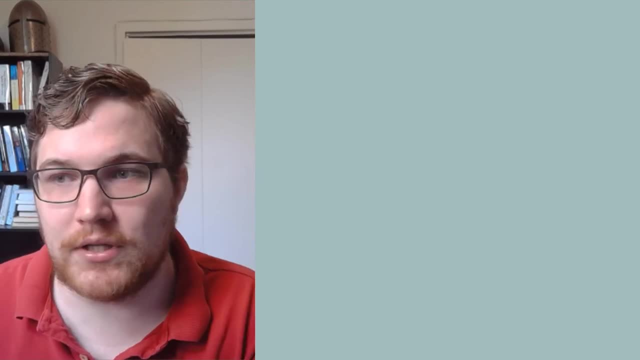 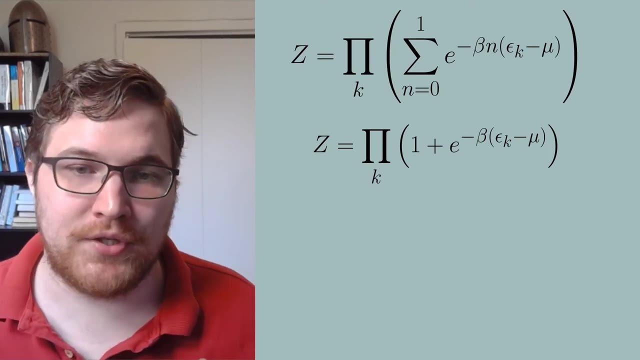 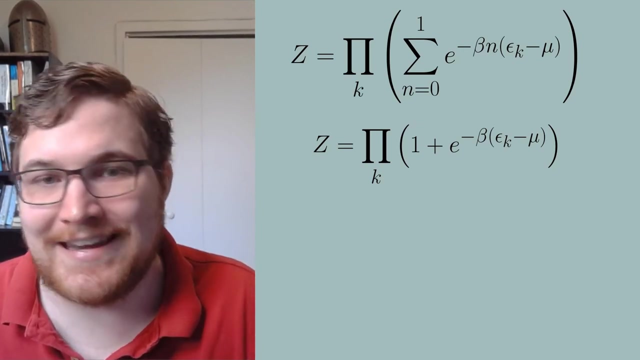 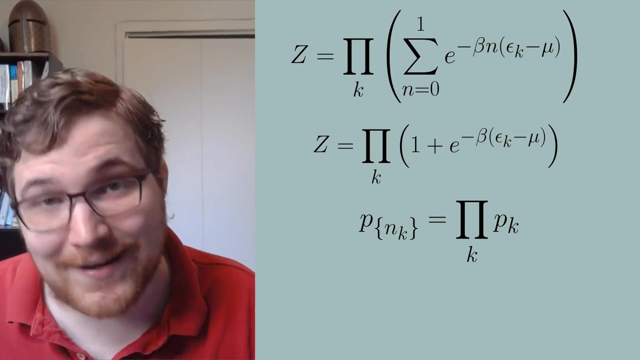 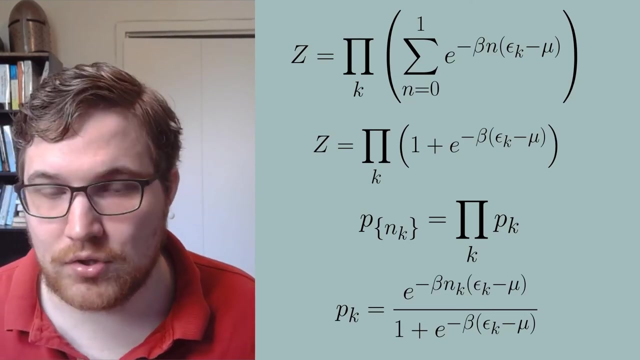 we can see that we can evaluate the sum quite trivially giving the following expression: This allows us to write the probabilities of a set of occupation numbers as just the product of probabilities for each individual occupation number, where these probabilities- p, subscript k for each individual occupation number- are written as the following relatively easy equation: 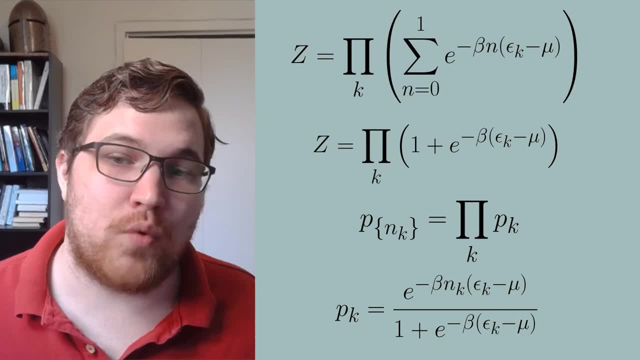 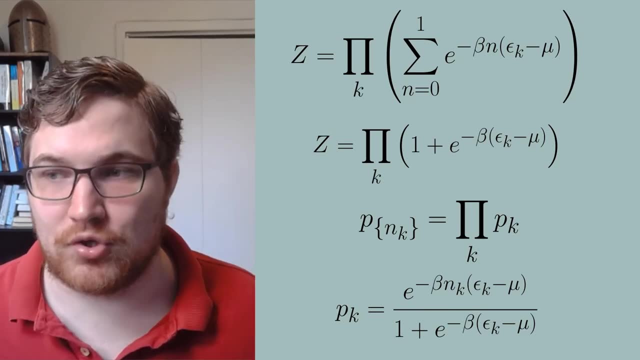 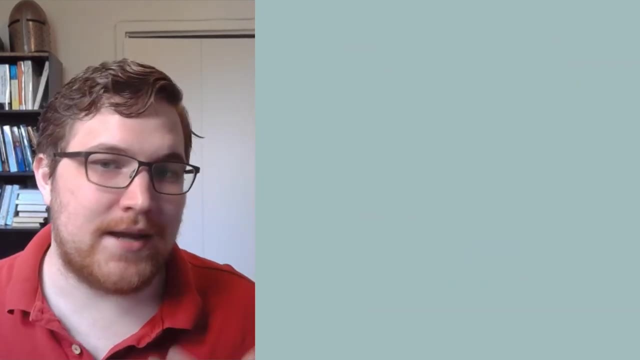 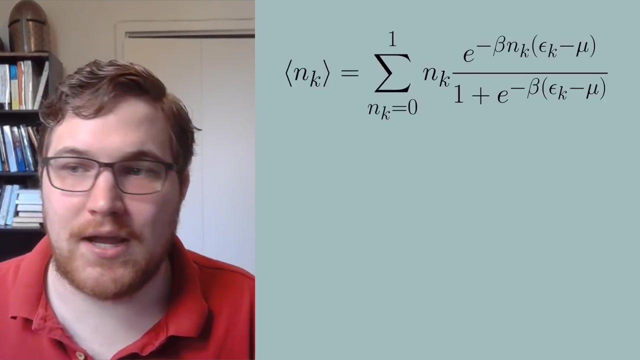 This then allows us to ask questions about properties and the possibilities of the individual occupation numbers, without appealing to the bigger picture, as each occupation number here has its own probability distribution. So we now have the goal of the video at hand: We want to know the expectation value of a single. 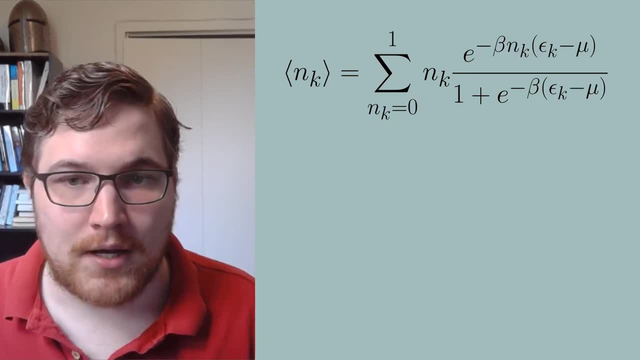 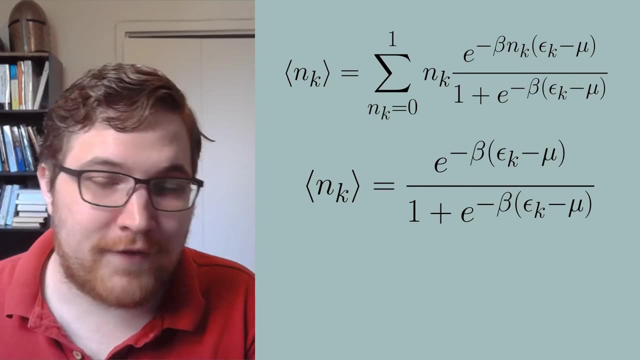 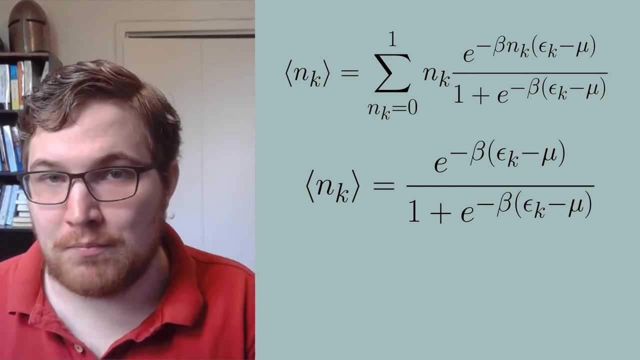 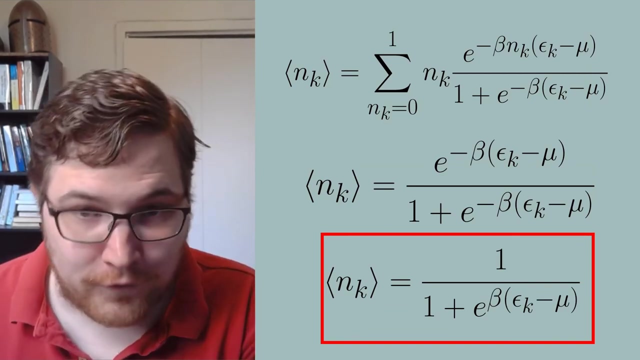 occupation number, as seen here. Evaluating this sum is very easy and we get the following expression: If we factor out the numerator and distribute it to the bottom, we get an expression that perhaps might look familiar to you, called the Fermi-Dirac distribution. The Fermi-Dirac distribution plays a 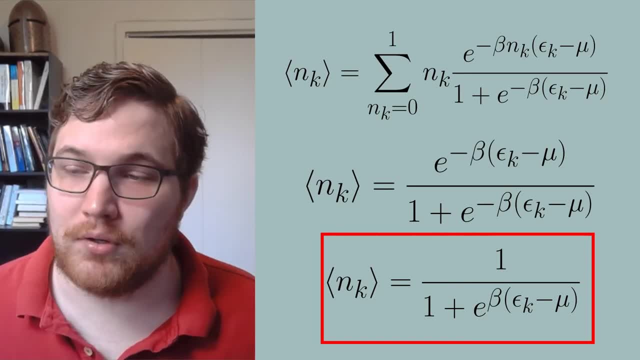 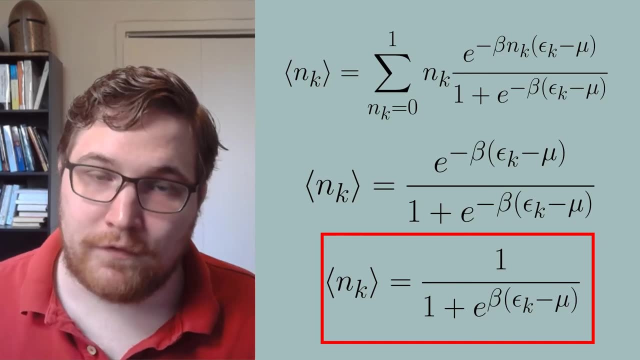 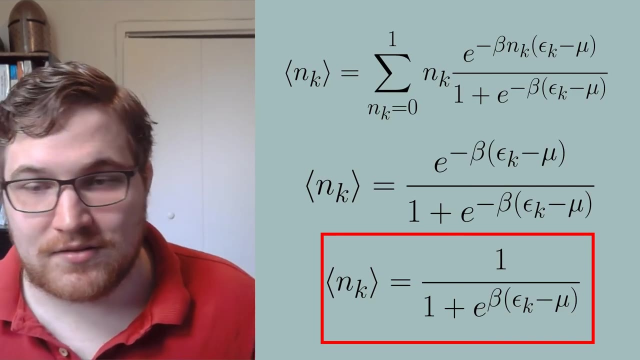 central role in our understanding of metals, for example, and is definitely a major triumph of statistical mechanics when applying quantum mechanical phenomena like the polyhedral Exclusion principle. In a future video, we will probably discuss the theory of metals, and this will definitely be a helpful starting point. 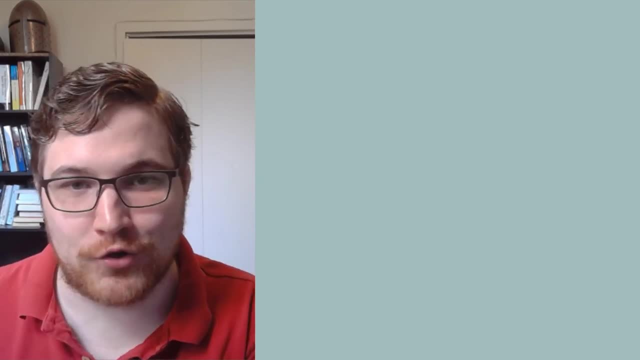 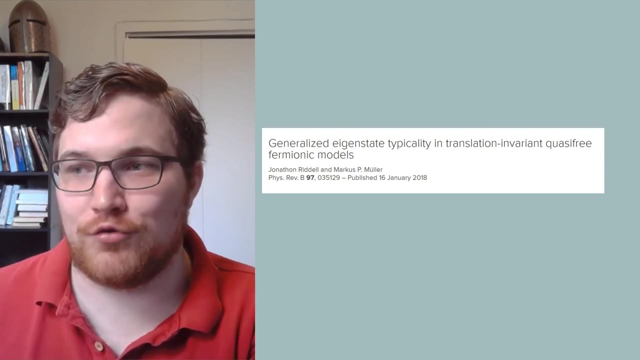 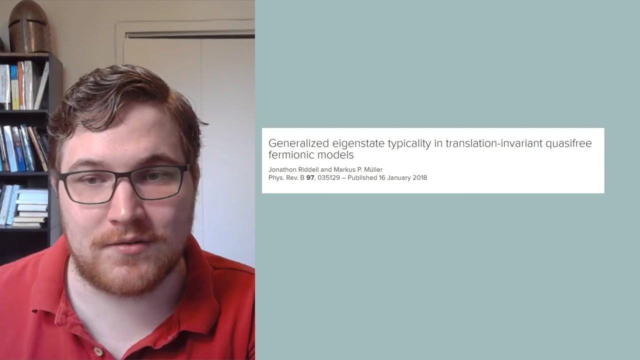 An interesting side note is that my first research article, my supervisor and I derived a generalized form of the Fermi-Dirac distribution in the language of the so-called generalized eigenstate thermalization hypothesis. Perhaps that'd be a fun video to make at some point.